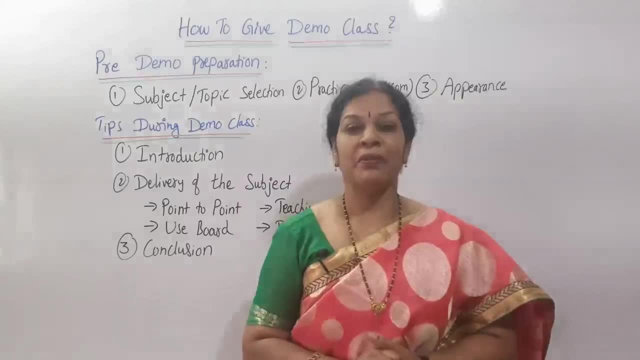 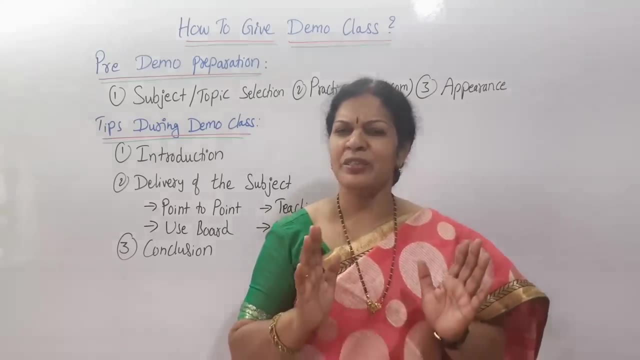 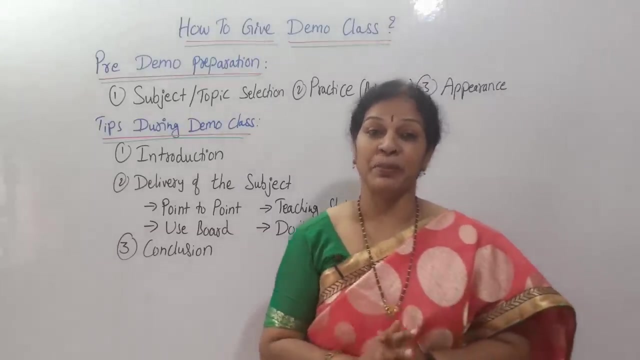 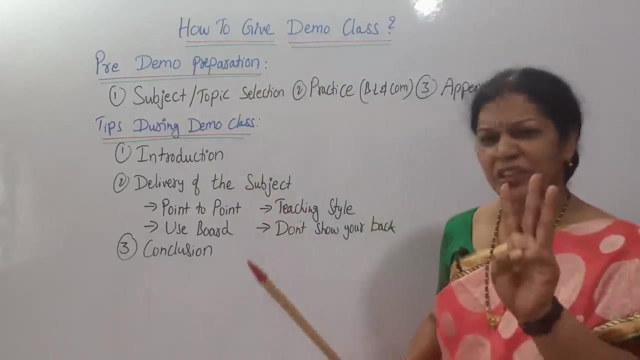 You can give a very good, wonderful, powerful demo class. Nobody can say no. So in that way you can give demo class. Let me tell you simple tips. The first thing is that pre-demo preparation: Before going to the demo class, you need to have some preparation. That's called as pre-demo preparation. Okay, So, as per this pre-demo preparation, only three points I wanted to say. First one is that subject or topic selection. 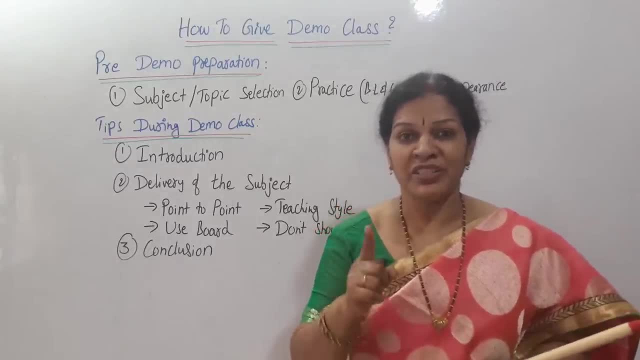 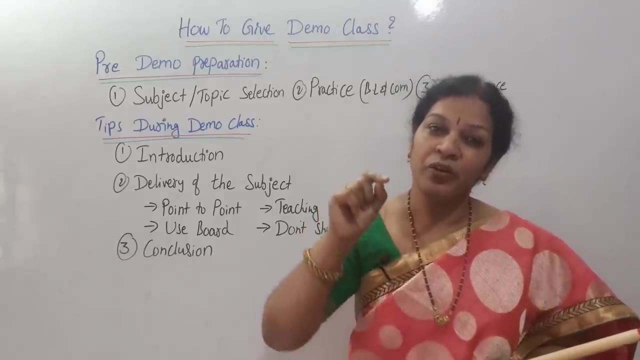 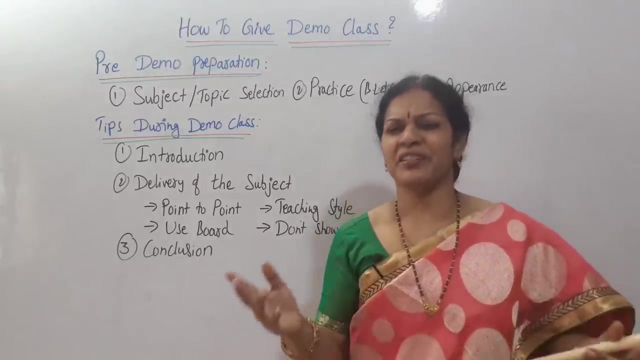 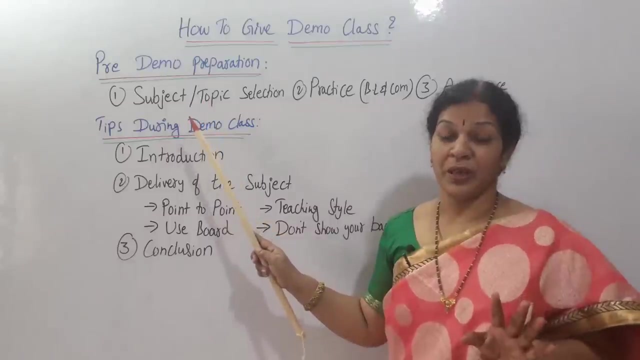 Going to play crucial role, Very important Which subject you have chosen, Which topic you have chosen. That's important Always. please choose your favorite topic, Your favorite subject where you have a lot of command. This is my topic. I can say very easily, without any hesitation. I can express So in that way. you have to choose the subject or topic, But make sure that you are very much, not just 90 percent, 99 percent, 100 percent. You have to choose the subject or topic. 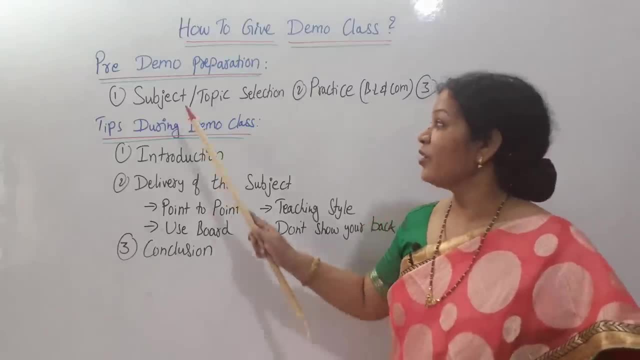 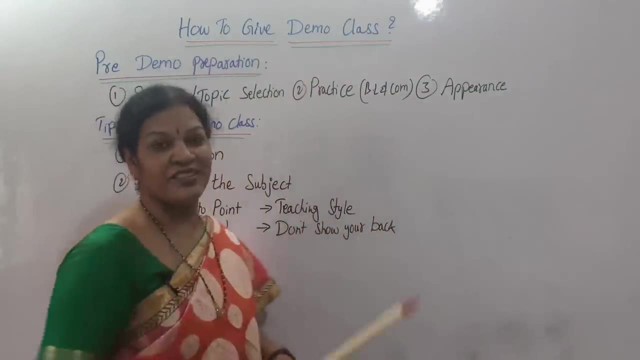 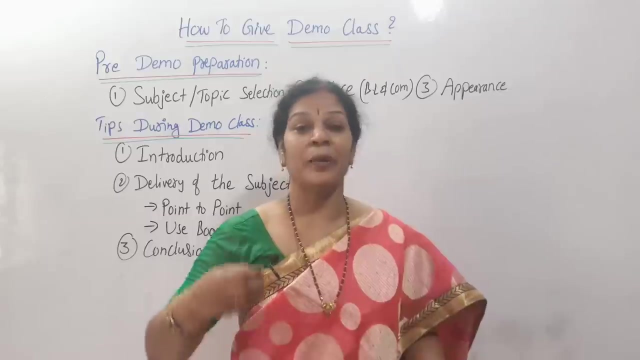 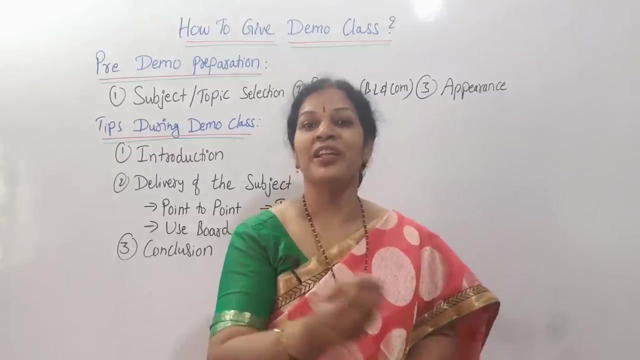 You must be sure about that topic. Okay. So this is important. Choose it before going to the demo class. Choose it Then. after that, what you have to do is your practice Same topic. Take piece of chalk, or stand in front of mirror and practice it, Explain it, Assume it Students are in front of you. Now I'm in front of camera, but I'm assuming that many teachers are in front of me. So, in that way, assume and practice. 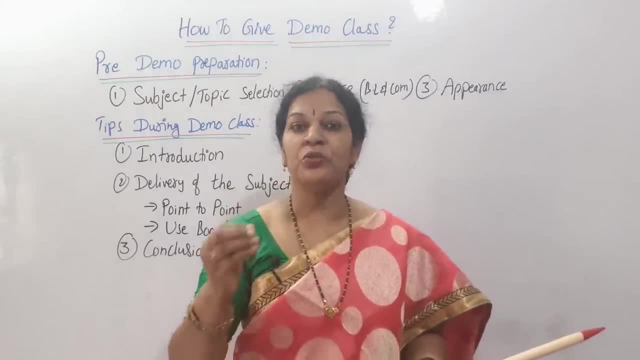 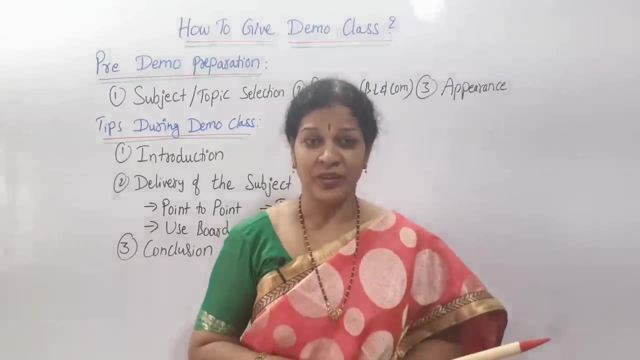 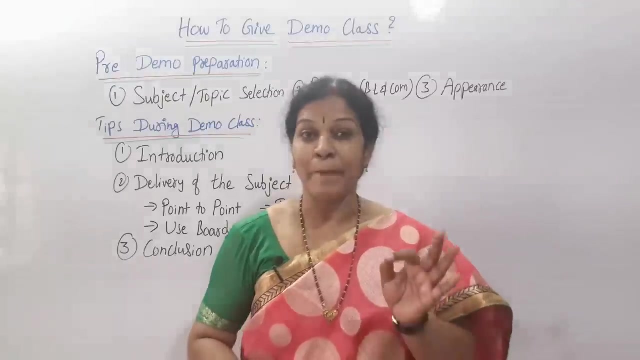 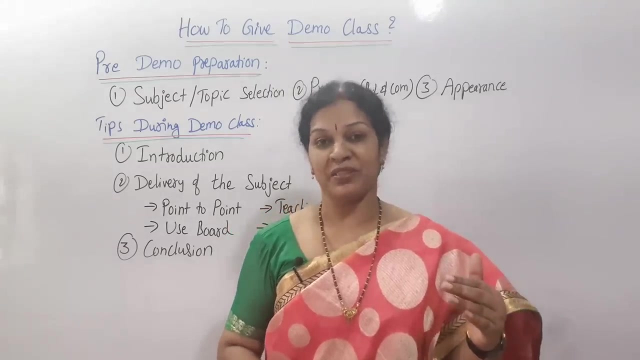 In front of mirror. Nowadays we have very good technology: Use the cell phone, Record your lecture and give suggestions by yourself or take suggestions from somebody who can guide you. There's a mistake is that you have to actify it like that You can take suggestion from others also. But practice makes you perfect. Practice will give you a lot of confidence. So go for practice many times, Okay. And next thing is that, while doing this, practice body language. 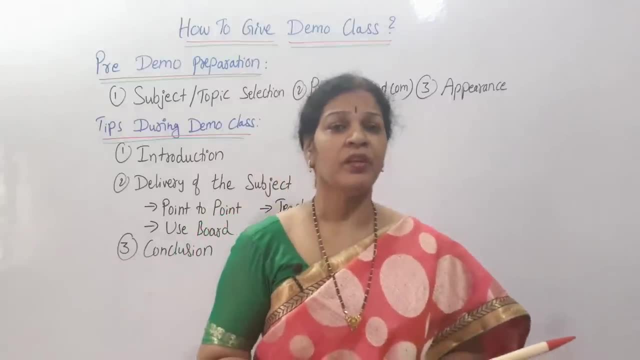 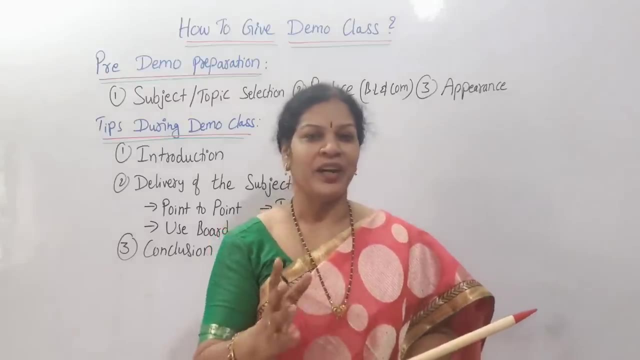 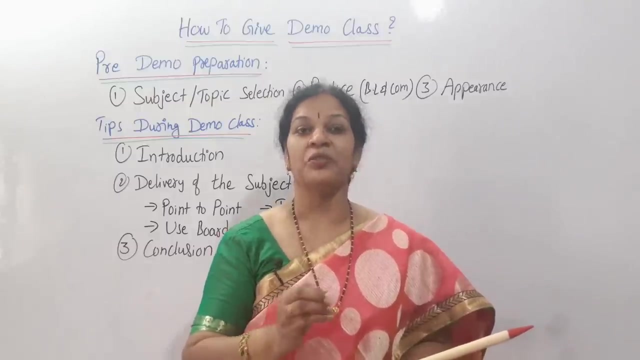 body language and communication skills plays a vital role. Communication skills: What we are speaking, students must understand clearly. For that, speak always good language. easy pronunciation, Use easy words, Don't use jargon words, because they are students Right. So always communication skills. clear, crystal clear, crisp language. Use it, And in communications also. we can do a lot of wonders. 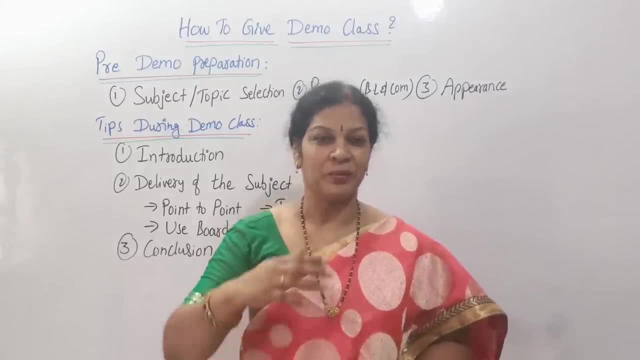 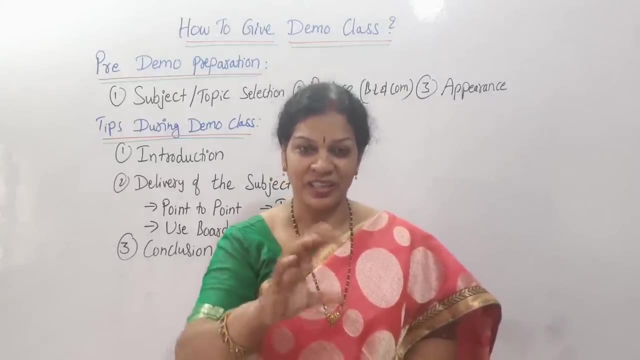 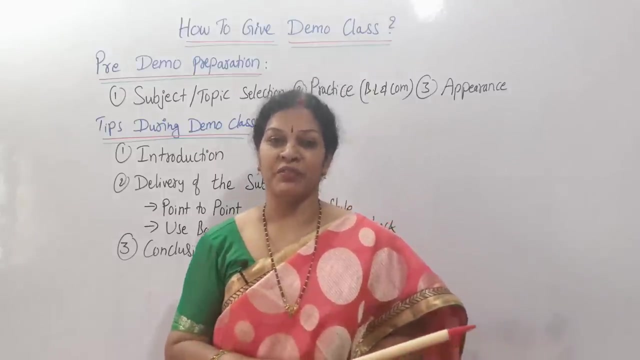 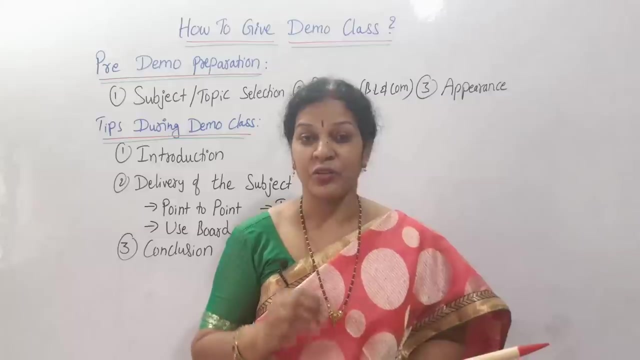 Like sometimes modulation of voice, sometimes giving a pause and sometimes asking them question through your talk, Like in communication, we can do some kind of modulations like this. Okay, So this is about communication and coming to the body language, It's also very much important Before you speak, your body language expresses about you what you are, So related to the body language. the moment when you go to the demo class, always practice. 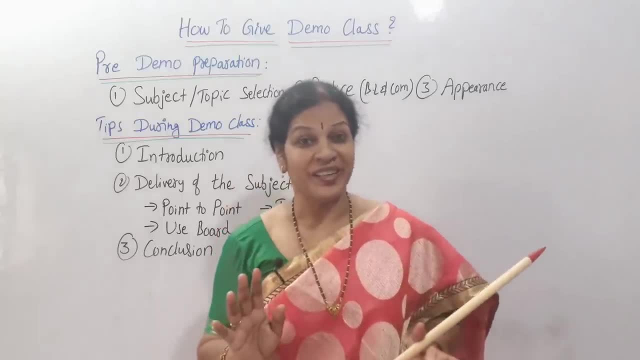 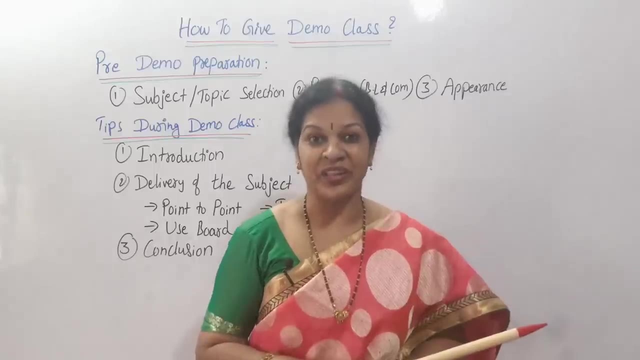 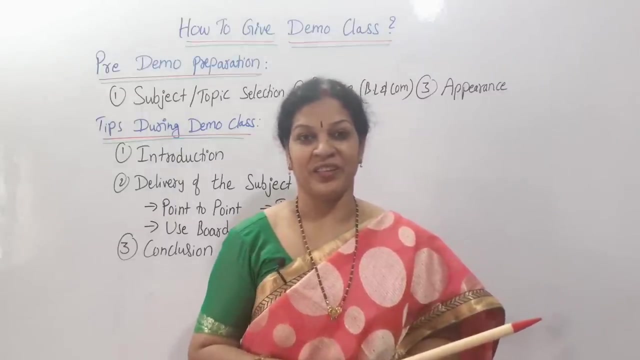 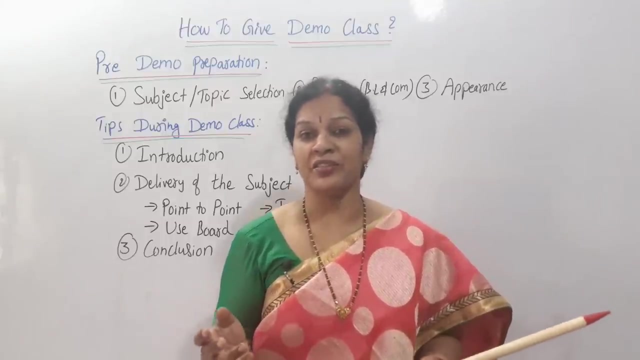 Please see that pleasant face, cool, a teacher, confident. that kind of facial expressions you have to maintain And also eye contact To whom you are speaking. make them a genuine confident eye contact. Smile, eye contact- These two are enough in the facial expressions And also when you use the hands. if the body is here, you can use comfortable moments like this. 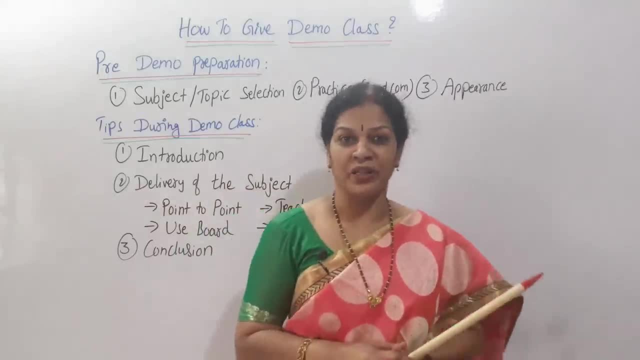 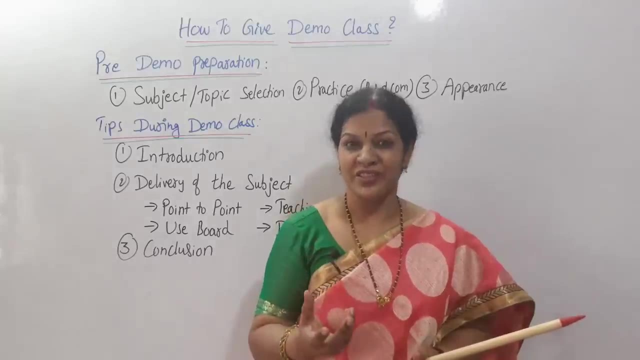 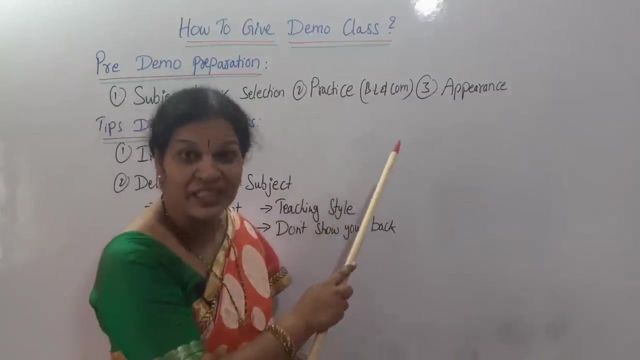 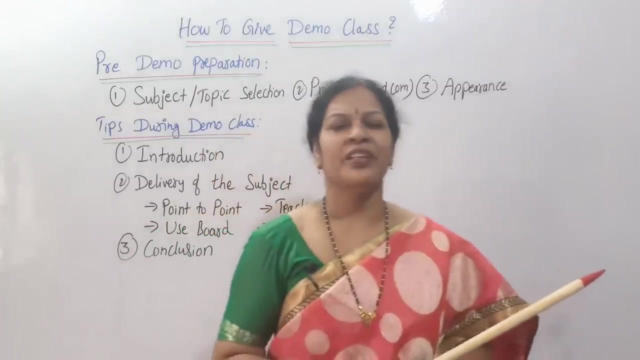 You can express it. Okay, So need not to stand at one side only and explaining: Okay, So that's the body language. Stand straight and look straight. Okay, Speak confidently, whatever you know. So these two things you have to remember while practicing only body language and communication skills. And next to third thing is that appearance A teacher should have always decent and decorum appearance, That is must. 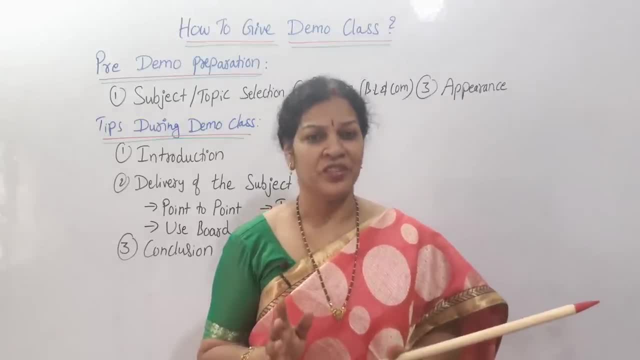 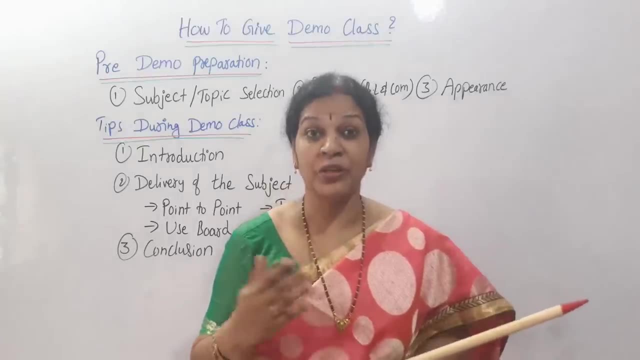 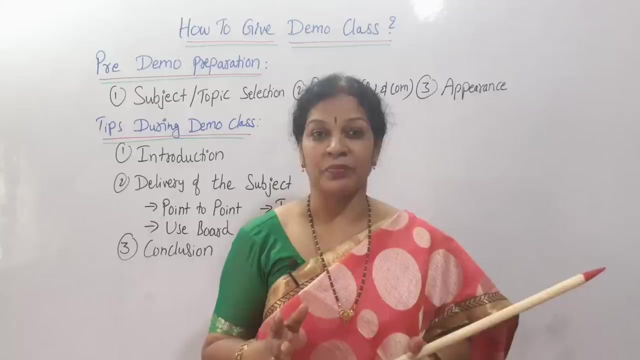 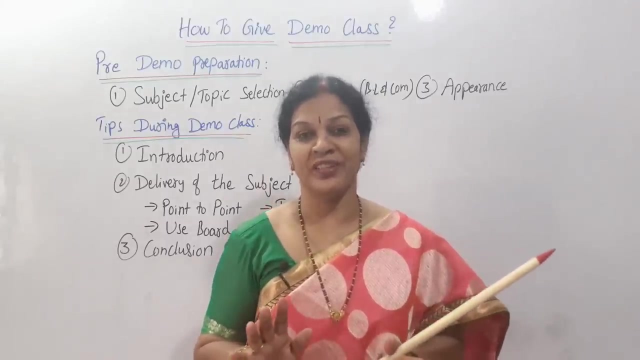 So always wear decent colors, decent, traditional, and a teacher must be like this as per your country, as per your location where you are teaching. If you are teaching in traditional school, you must be. If you are going to international schools, observe the custom and observe their whatever they required. So according to that, your appearance should be always decent and pleasant. It doesn't mean that you should look smart. 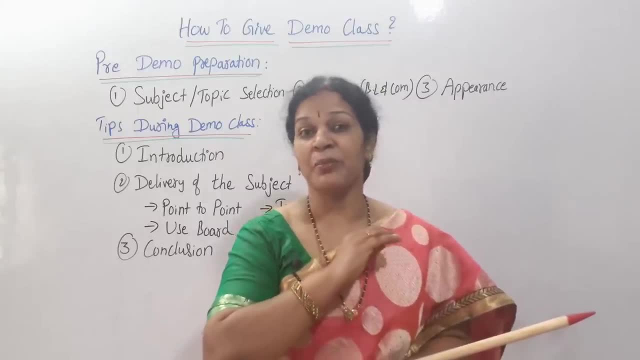 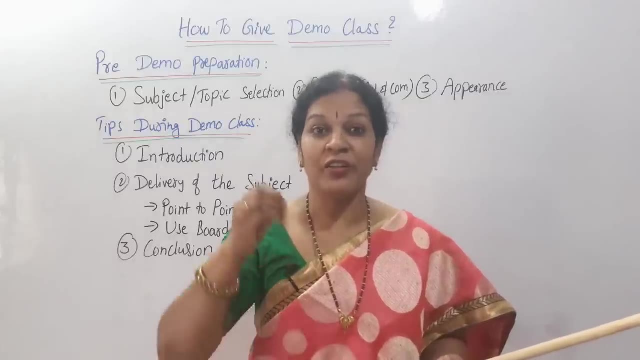 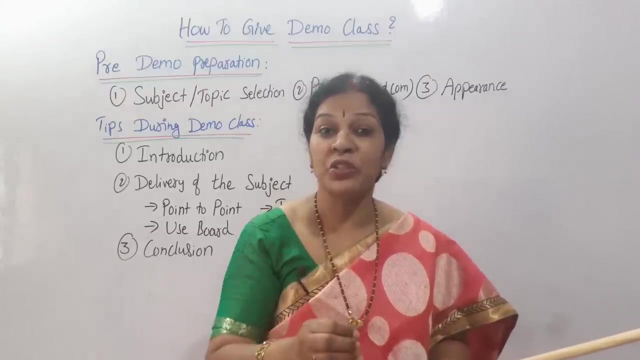 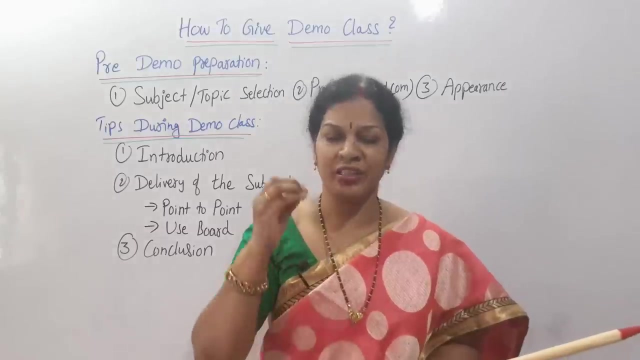 It is different For teaching field. smartness doesn't matter at all, Looks are not going to matter. What is going to matter is here your subject, your explanation and your command and the way you teach, the way you attract the students with your subject. that is going to matter. Short height, lean, thin, dark color doesn't matter at all. Please ignore this kind of things from your mind, Because in my career I have seen many teachers. 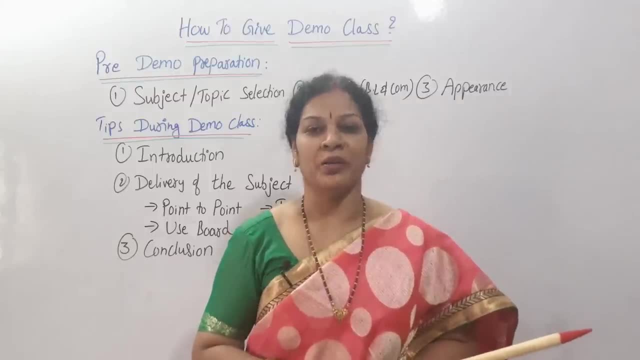 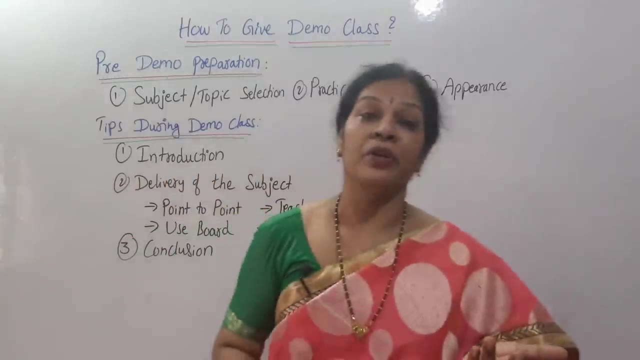 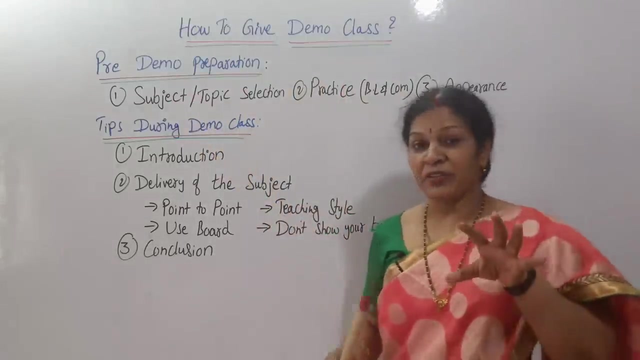 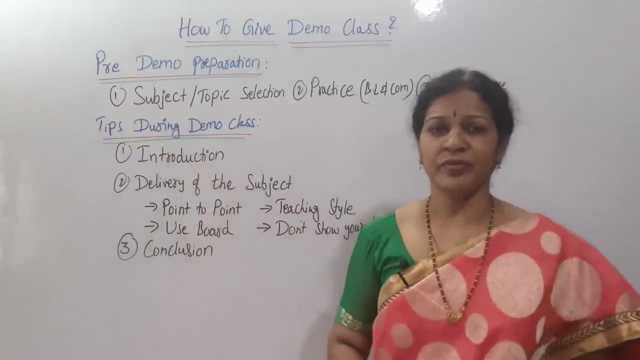 Many lecturers, many professors, looks are not going to matter at all, So please remember this. but decent appearance, These three things. you just have to prepare it before going to the demo class, at least one week before you start it: Subject, topic selection, practice and appearance. Then after that, during the demo class, what you have to do. this is tips during demo class, Simple three tips. The moment when you enter into the demo class, introduction is important. 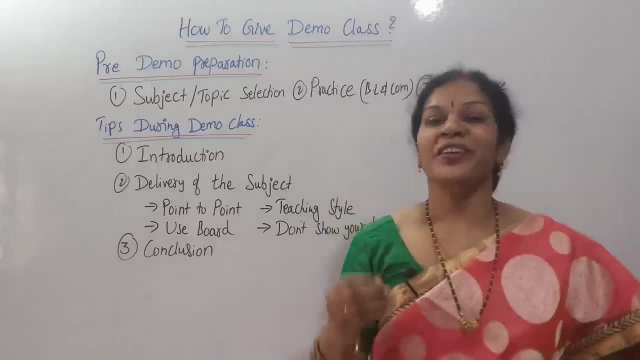 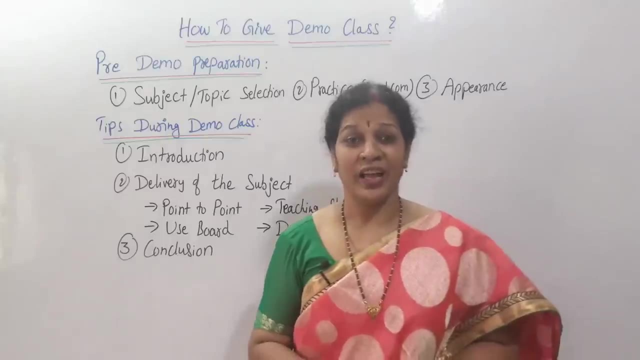 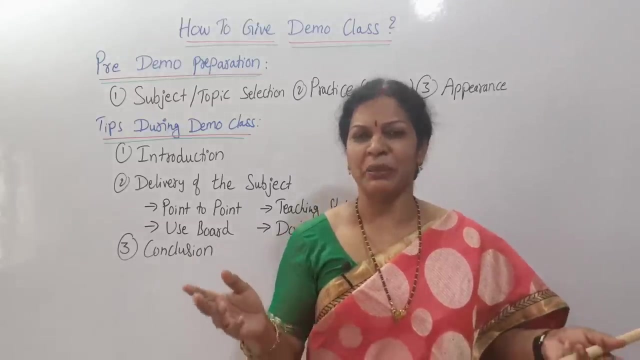 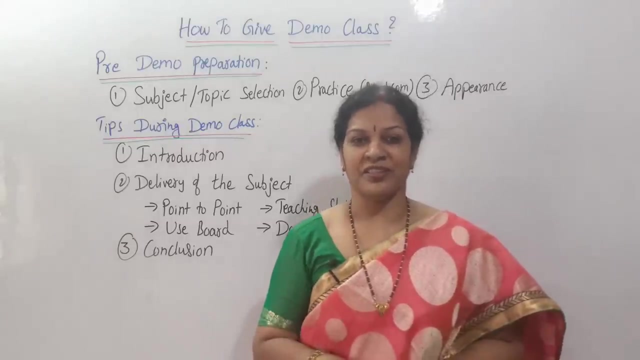 We won't teach subject right. So the moment when you enter, coolly, comfortably, take a position, stand in front of board, take a piece of chalk and give your introduction. Hello everyone, Good morning dear students, Good morning everyone. Whatever may be, whatever you are, that is. salutation is important. After that, introduce yourself in just two to three sentences, Just like as I'm going to give you the myself introduction. Good morning everyone. 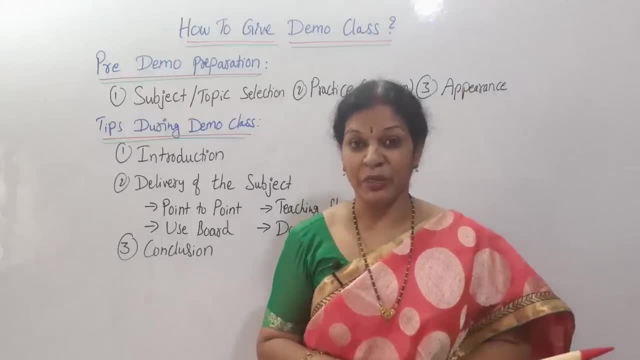 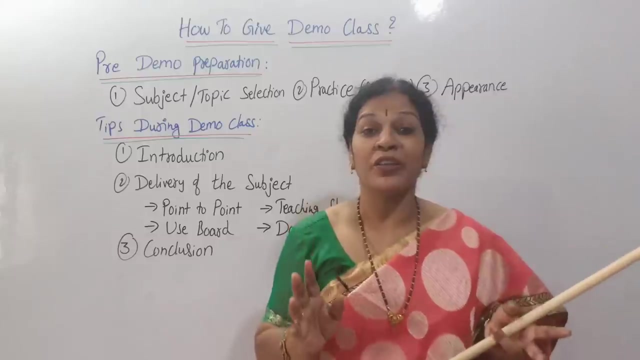 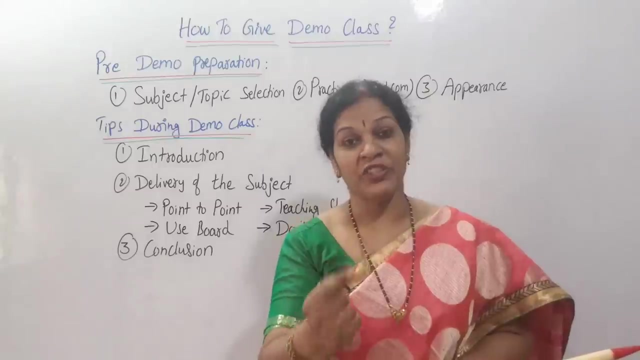 Hello everyone. This is Dr Devika Bhatnagar. I'm going to tell you about cash flow statement. This is one of my favorite subject. Many people say that this is tough subject. Not at all. It is quite interesting. My favorite And I'll make you to understand- just to 45 minutes. Focus with me. This is my self introduction Means. I gave my introduction and also which topic I'm going to speak. I gave a conference to the students that this is not a tough subject. 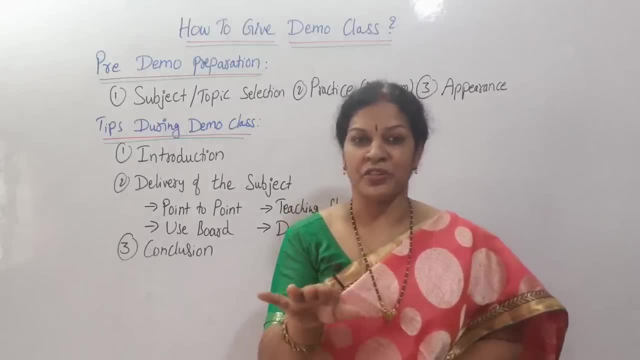 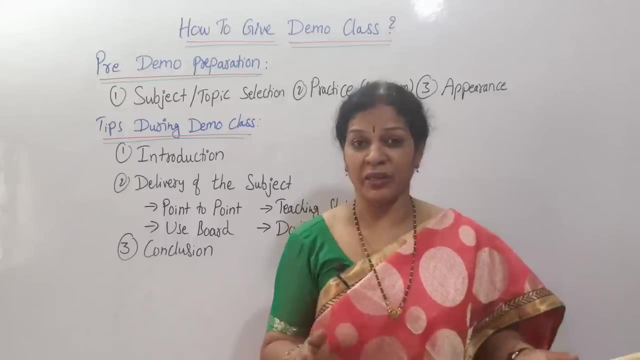 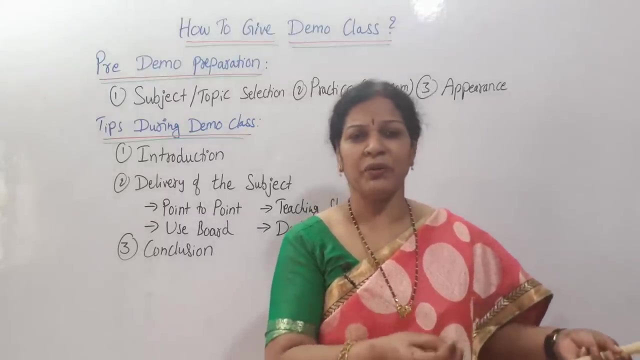 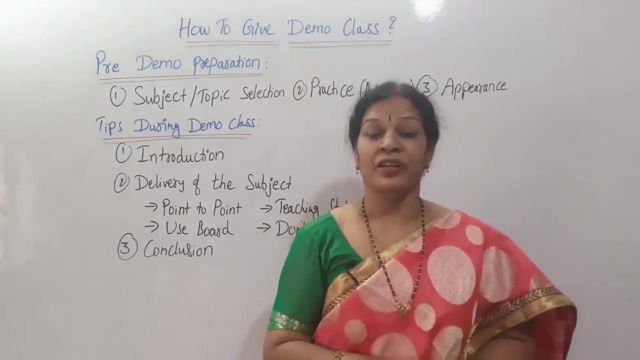 So in that way, self introduction, first introduction, Speak about your name and you can speak about your qualifications Also. I have done so and so I have done MCom, MBA, MPhil, PhD. What my qualifications? I have 25 years of teaching experience, And if you have five years, 10 years, whatever it may be, So that teaching experience also. please introduce yourself There itself. only you can take this points. So that's about your introduction. 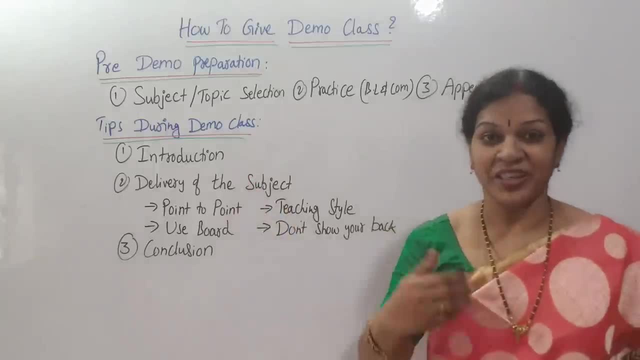 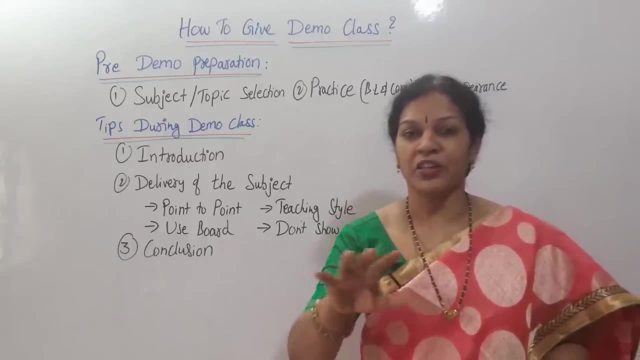 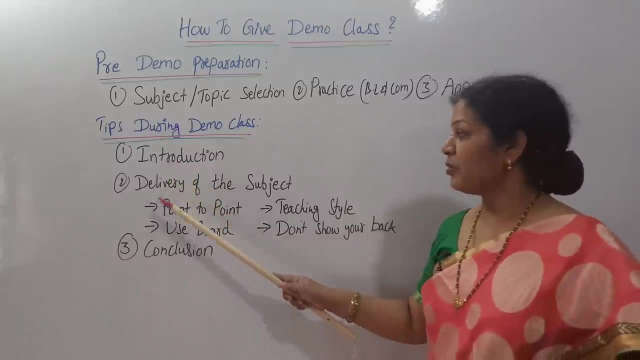 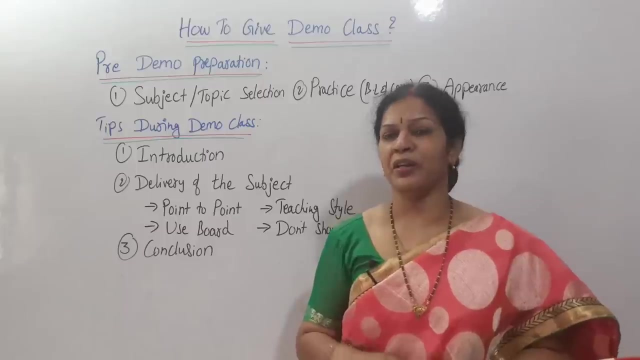 After that, what to do? So delivery of the subject, Getting into the subject. So when you take up that topic, particularly please remember, don't rush up, Cool, Be cool. Explain point to point, Step by step. you have to explain- So this is important- Point to point, step by step, Like if you take any topic. that introduction I wanted to give any kind of what do you say? definition. 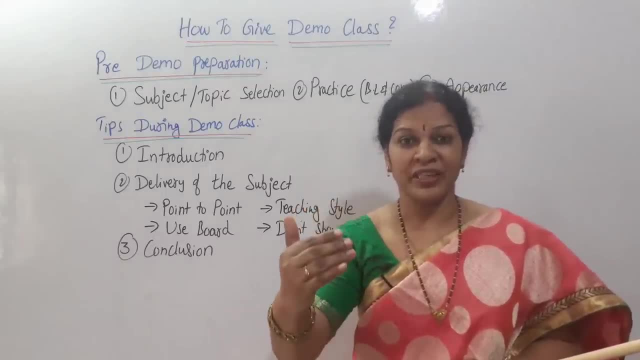 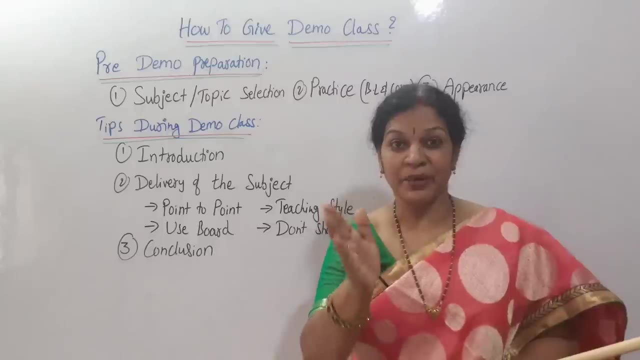 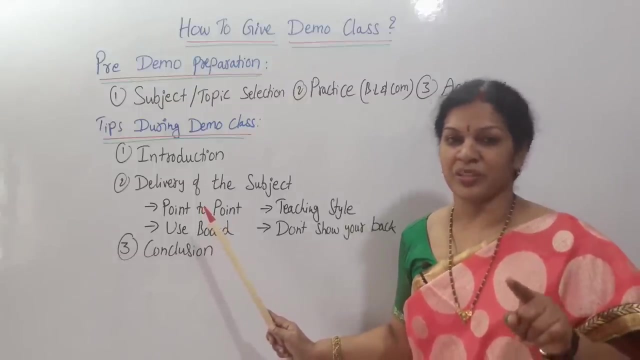 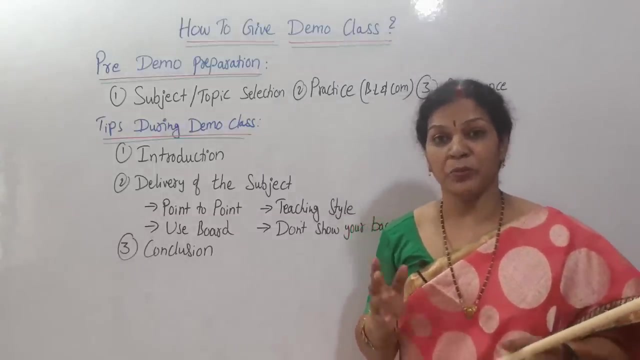 Or formula. That is introduction part. Then after that, giving a depth information, Getting into the deep of the talk. Then after that, conclusion, Like step by step, you have to go. So this is you remember coolly. explain That already. you have practiced, you can explain. This is about point to point explanation. Then after that, teaching style: Your teaching style also going to makes a lot of matter How confidently you are speaking. So what is your body language? 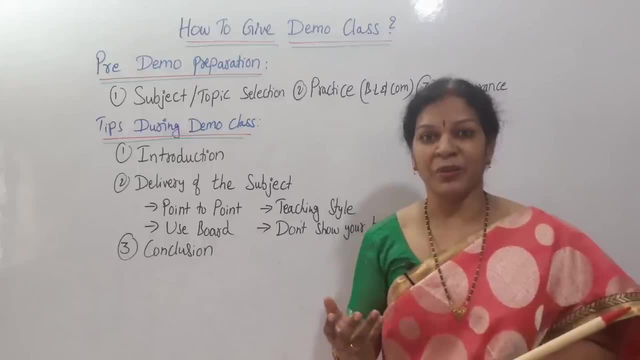 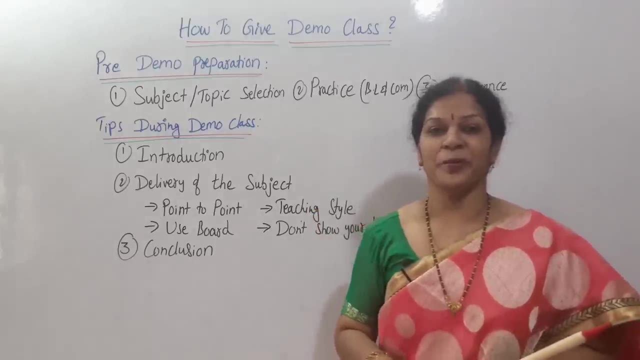 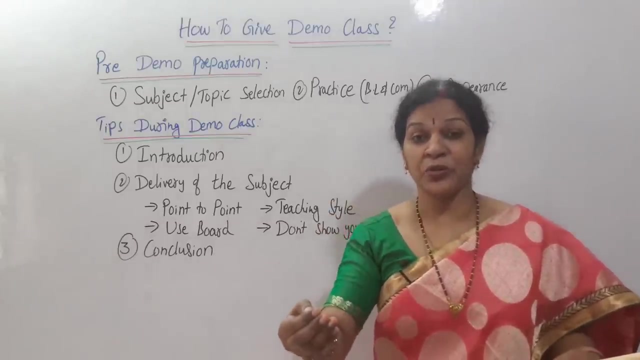 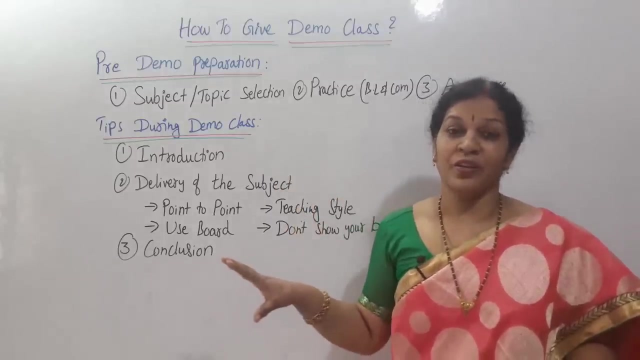 How you are speaking, What is your teaching style? So how you are communicating. So all these things comes under the teaching style. Confidently speak, Do not worry about anything. What is going to happen, Whether they are going to select you or not, What questions they are going to ask, All these things keep it aside. Nothing should come inside of your mind. Only your focus should be on that topic. So have a good teaching style. Practice it, You'll get your own. You'll get your own teaching style. 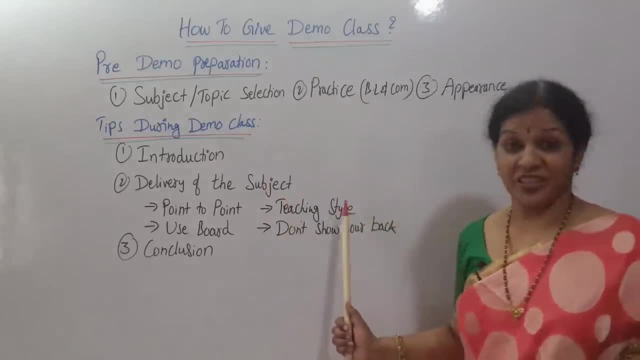 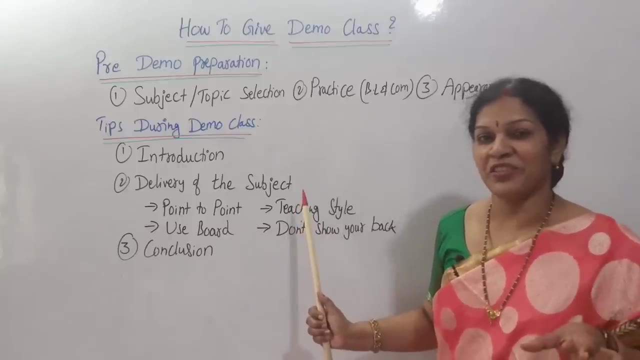 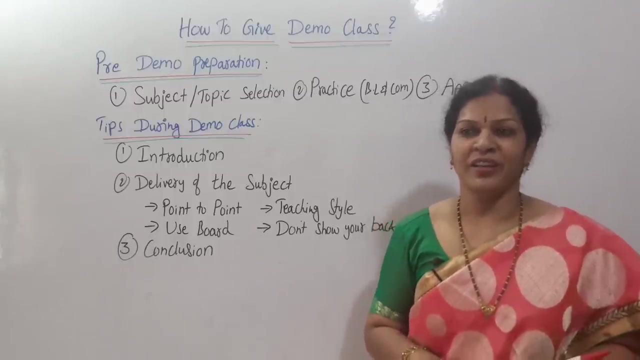 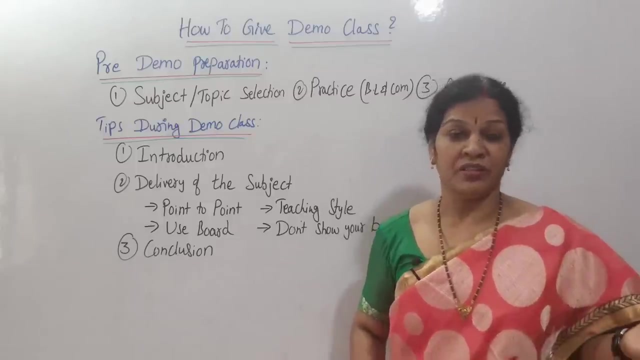 Unique style, Need not to copy anyone. So that's about teaching style. Mannerisms also going to matter. So how do you explain Body language, communication skills? subject: explanation: All these things comes under the teaching style. Maintain a good teaching style Once if you have own style. wherever you go- whether it's a demo class, or maybe you are giving a lecture, maybe you are delivering a seminar, whatever it may be- the same thing is applicable. The same tips are going to be useful for you. 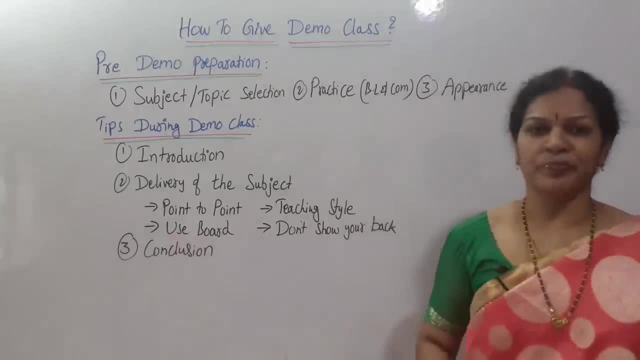 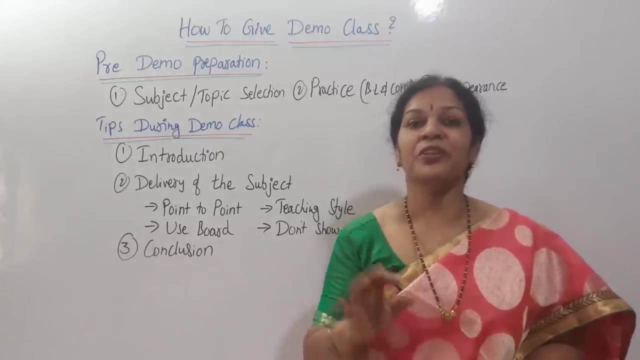 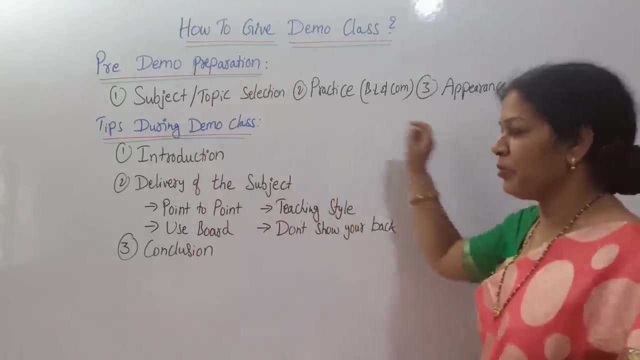 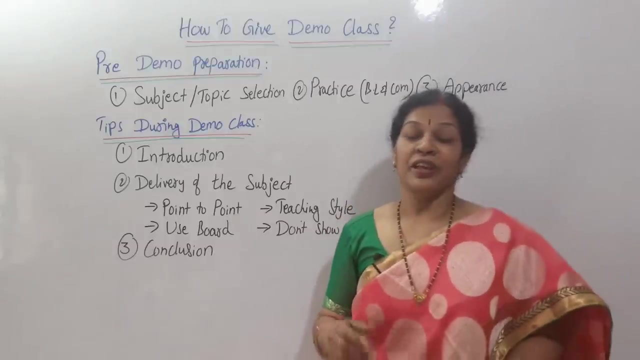 Okay, That's about the teaching style. Next, one use board. Sometimes, due to fear or due to some consciousness, some teachers they forget to use the board. Use comfortably the board Maximum board from top to bottom, wherever you want. If you want, you can take the definitions, introduction part, any charts, diagrams, anything you want to explain. please use the board with a piece of chalk. 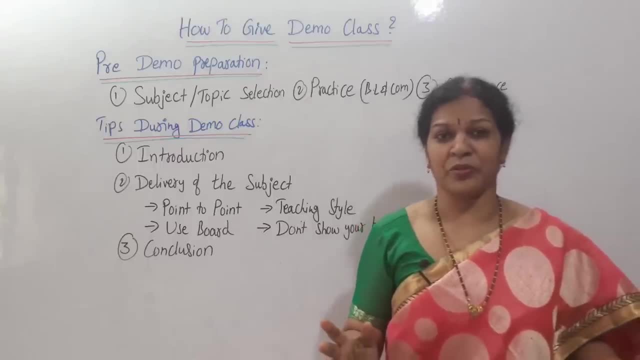 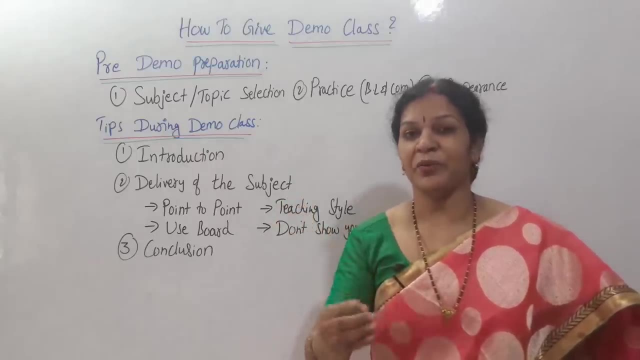 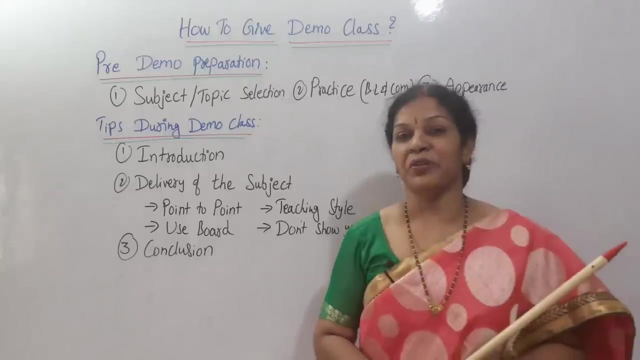 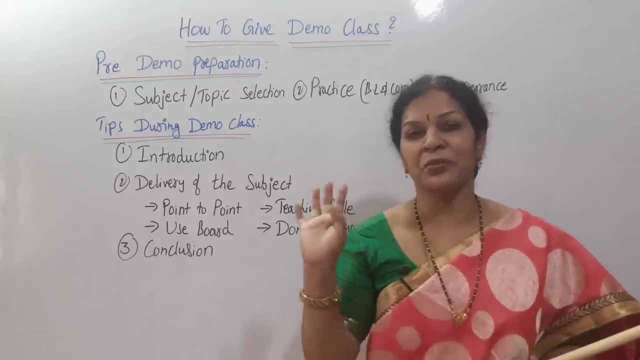 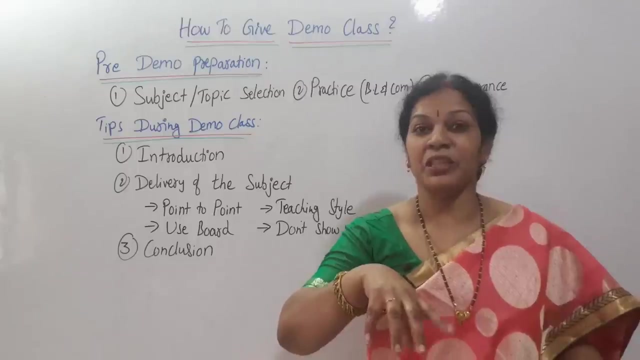 Okay, It's also acceptable to rub the board. also Rub it and once again you write it. Assume that students are totally involved in your talk. In that way, step by step, you can go. Just remember this: using the board is important. In one of the demo class I have observed, one teacher was giving a demo class. She has given a very good demo class, but she did not use the board Not even a single time. also, Simply, she was explaining, Then the board members of the interviewers. they were discussing among themselves. 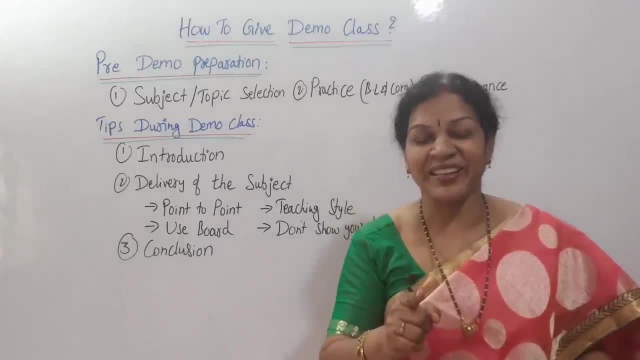 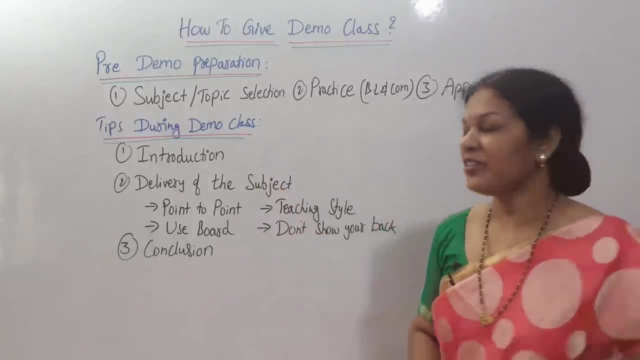 Did you observe that she did not use the board? That's a drawback. Please be careful, So use the board. Next one is that don't show your back when you are writing on the board. Some, especially some teachers and lecturers, they write like this. 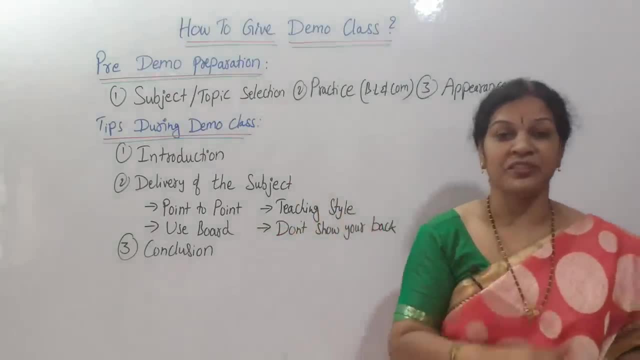 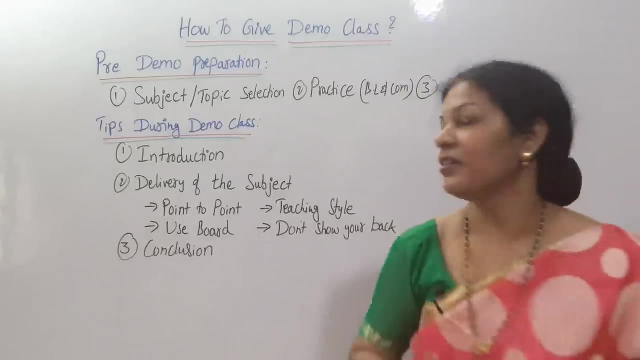 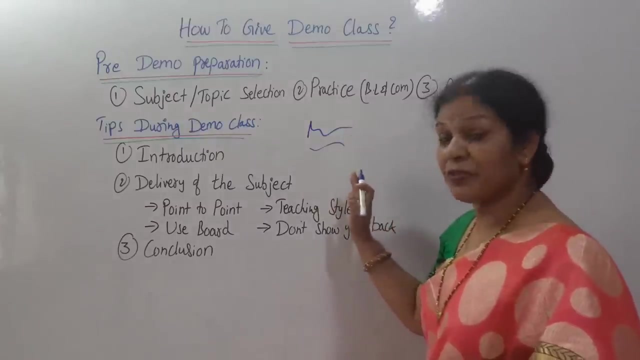 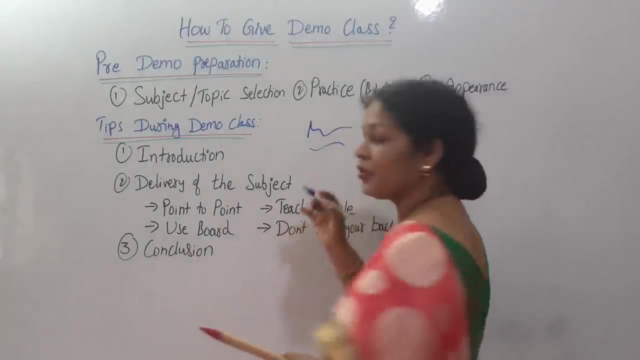 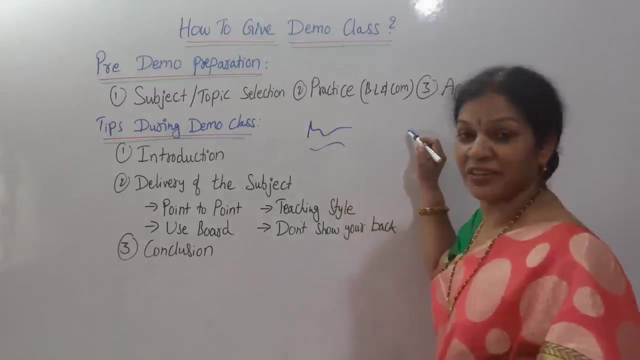 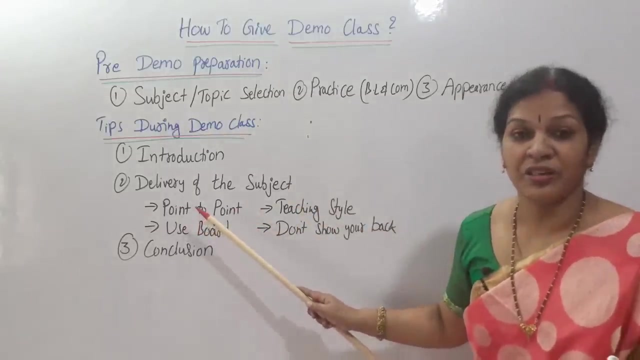 Showing the back. Never do this. This is a blunder in teaching field. When you want to write anything, so this is the position, So write it like this, whatever you want. So your position means 45 degrees. Okay, Half you are looking at the students and half you are writing. If I write like this, students can't see anything and it is going to give a negative impact. That is why, always, you have to write like this. This is very much important. Then, after that, these are the: simply delivery of the subject, During the delivering of the subject. Lastly, conclusion. How should be a conclusion? 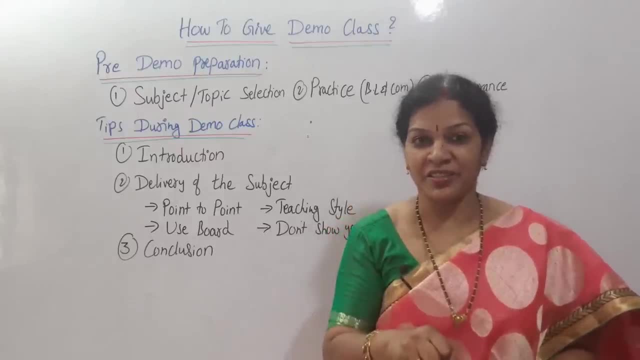 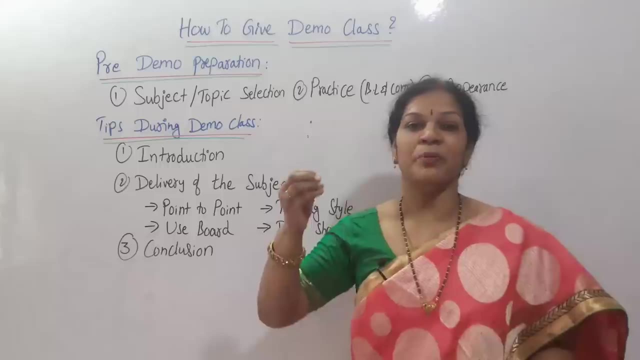 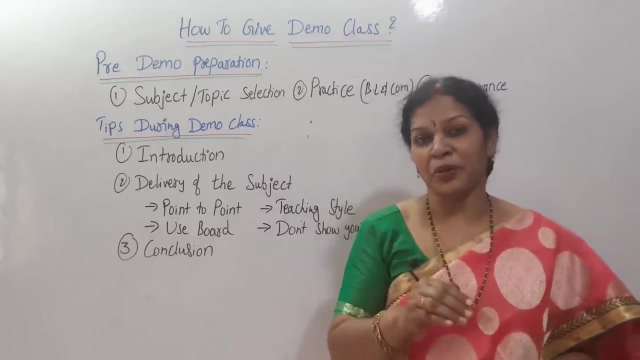 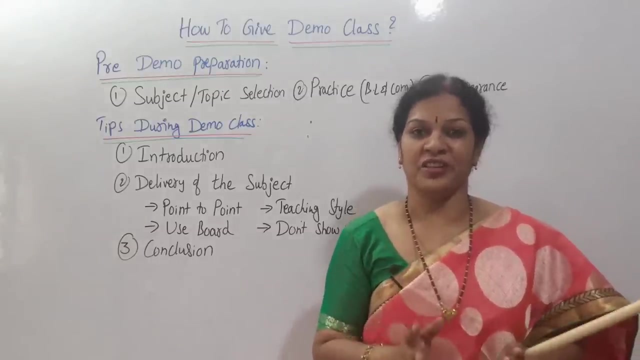 The entire talk, Concise it, Conclude it, Revise it, Gun points you take. This is what we have discussed. Let me give you in a nutshell, Let me explain the entire topic in just two minutes. Like that, wrap up the topic. Wrap up means condensing the total concept and you are delivering once again in a nutshell. So wrap up the topic. conclusion Then, after concluding your topic, 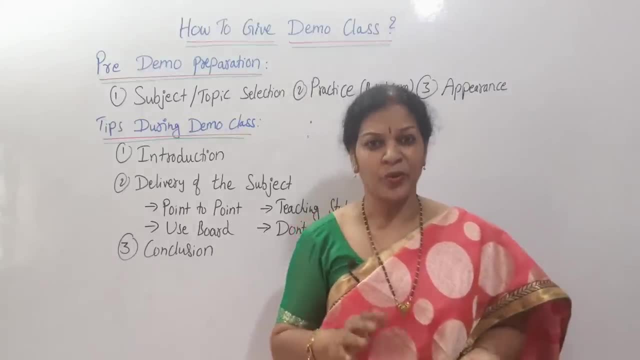 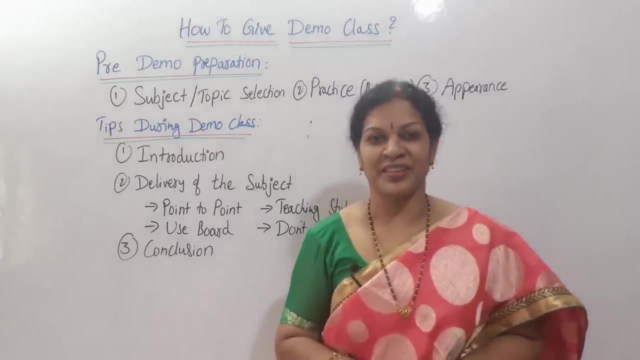 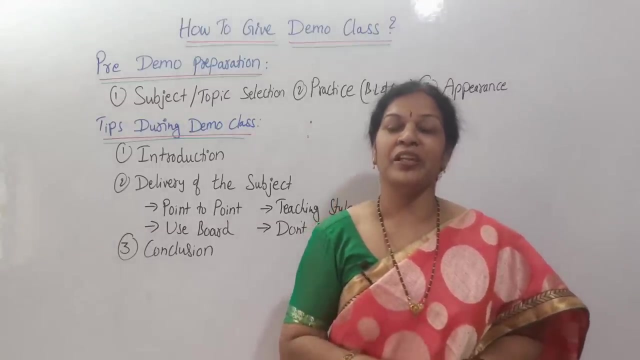 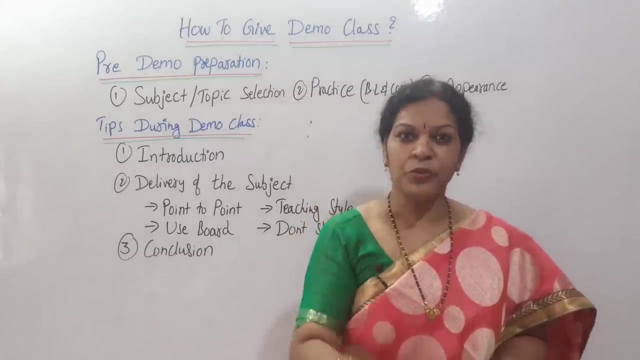 Then ask the students: did you understand? Hope the topic is clear. Is there any doubts? Please feel free to ask your doubts. Like you invite the students to raise the doubts also. That is the best way to deliver any talk subject specially. So after conclusion, you ask them and you give them a freedom to raise the doubts. So then, after that, thank everyone. Thank you everyone. 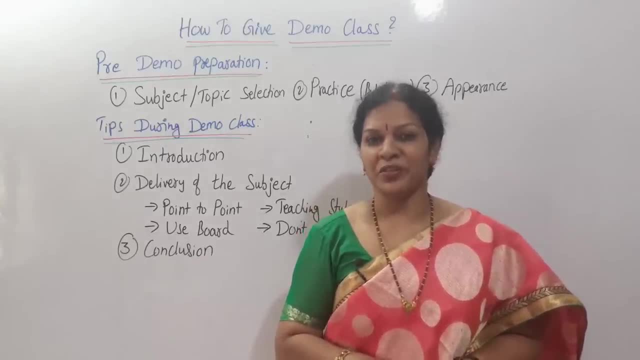 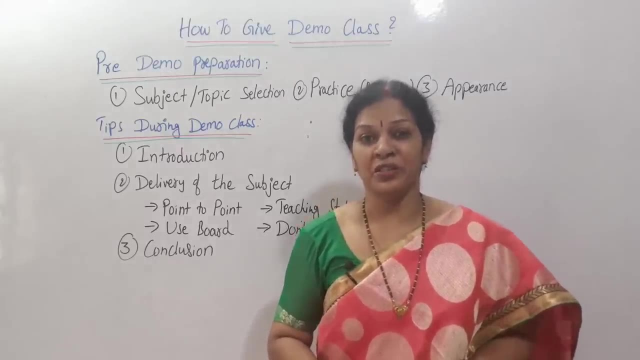 For your cooperation and hope the talk is useful. See you soon. Like positively, you are given demo, but you are expecting that you are going to be a teacher, You are going to be a lecturer, You are going to be a professor to that students. In that way, see you soon. 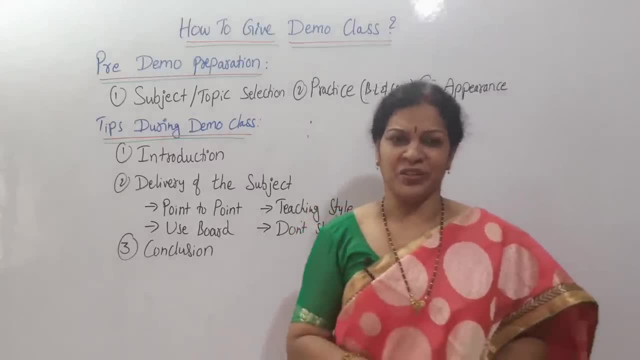 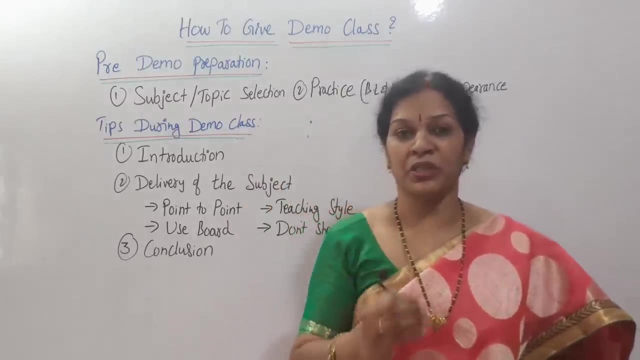 Take care of your career, Something you can. You use your own words. So in that way you have to give the demo Hope. I am clear. Let me revise it Whenever you wanted to give demo. first important thing is that pre-demo preparation.